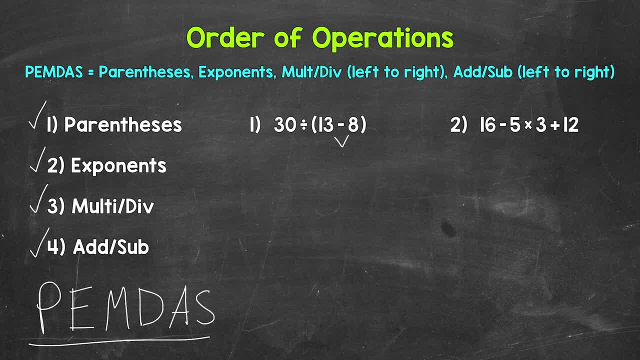 13 minus 8.. And then we have 30 divided by, and then in parentheses, 13 minus 8.. So we have 30 in parentheses: 13 minus 8 is 5.. Then we need to bring down everything we did not use. So we have. 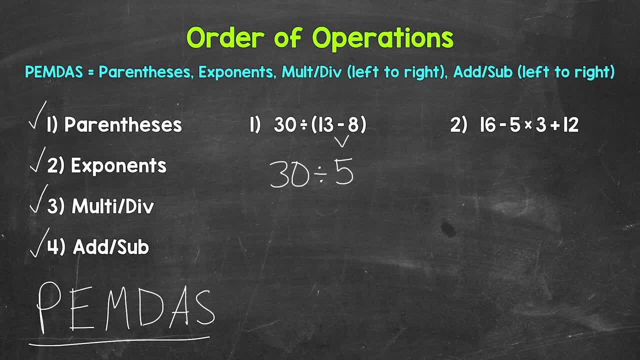 30 and then divided by 5.. So now we have 30 divided by 5.. We only have one operation here: division. So that's what we need to do: 30 divided by 5 is 6.. So our final answer: 6. So. 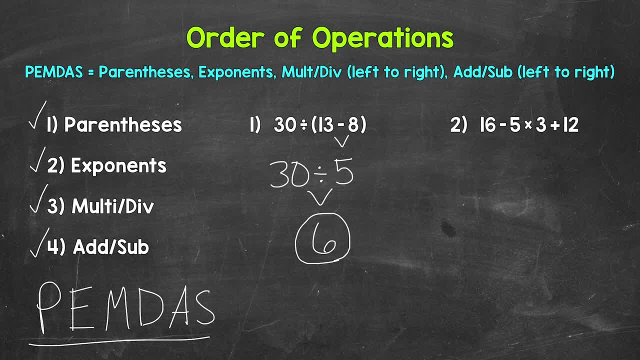 number one. we worked through the order of operations, So we have 30 divided by 5.. So let's move on to number two, where we have 16 minus 5 times 3 plus 12.. Let's work through the. 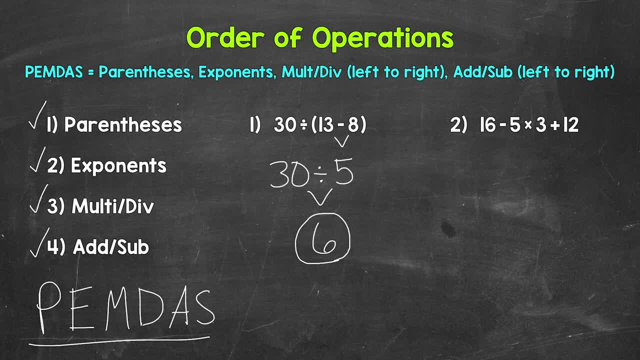 order of operations. Do we have any parentheses? No, So let's move on to exponents. Do we have any exponents? No, So let's move on to multiplication. So let's move on to multiplication And division. Do we have any multiplication or division? Yes, So that's where we start. We have. 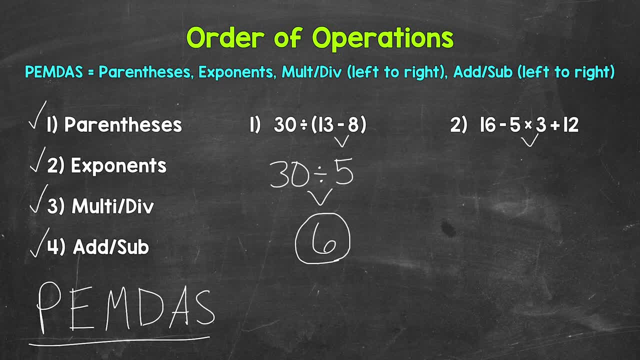 multiplication, We have 5 times 3. That is 15.. Now we need to bring down everything we did not use. So we have 16 minus 15 and then plus 12.. So we have 16 minus 15 plus 12.. And we need to. 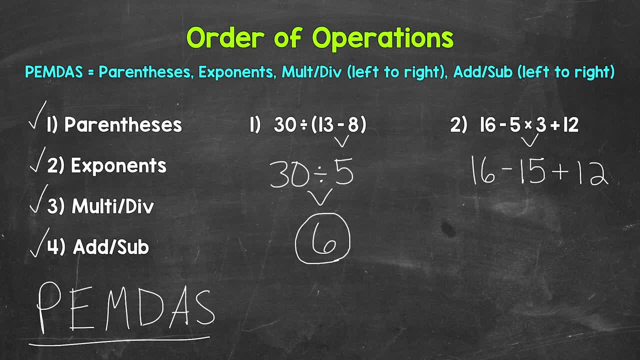 continue to work through the order of operations. So let's move on to number two, where we have the order of operations. Any parentheses: No, Any exponents, No, Any multiplication or division, No, Any addition or subtraction. Yes, We have both addition and subtraction. Since we have both, 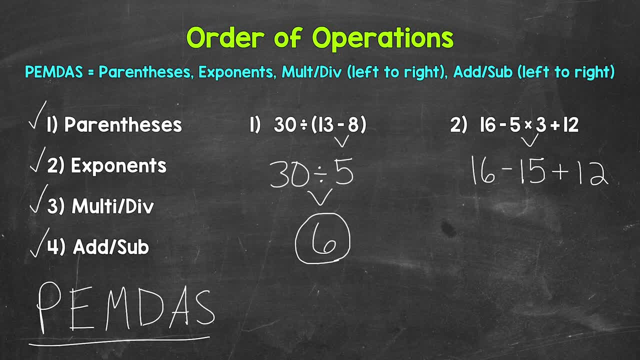 addition and subtraction. we need to work from left to right. Addition and subtraction are on the same level. They are the same priority in our order of operations. So again, we need to work left to right. When working from left to right, we need to do subtraction first here. So 16 minus 15. 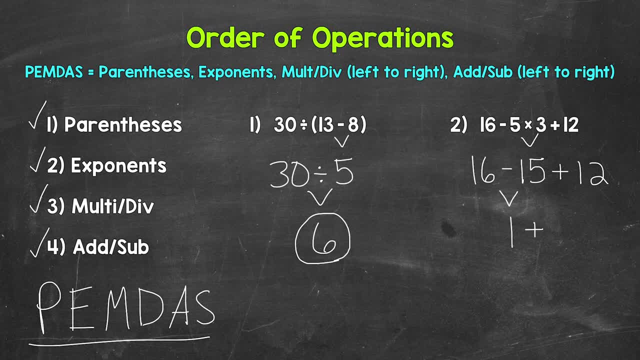 is 1. Bring down everything we did not use, So plus 12.. And now we have 1 plus 12.. We only have one operation left. So that's what we need to do. We need to add: 1 plus 12 is 13.. And that is our. 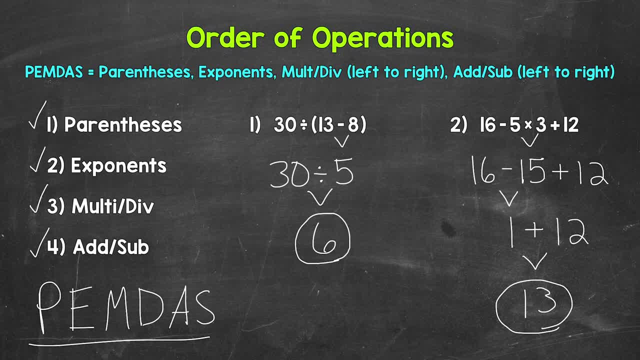 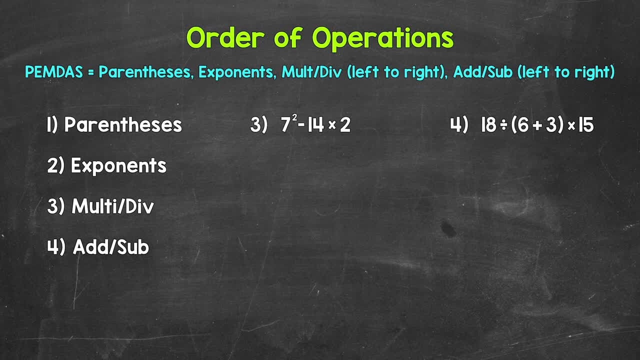 final answer. Let's move on to numbers 3 and 4.. 4.. Here are numbers 3 and 4.. Let's start with number 3, where we have 7 squared minus 14 times 2.. Let's work through the order of operations. Are there any parentheses in this expression? 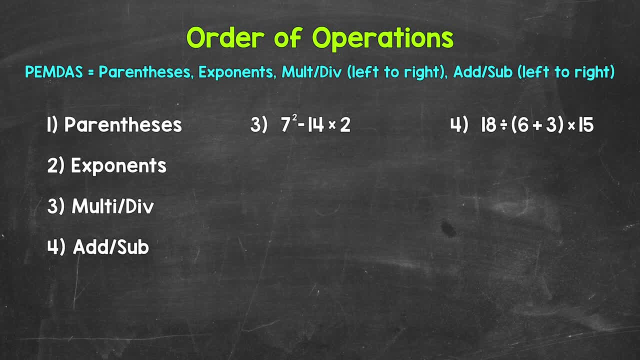 No, So let's move on to exponents. Are there any exponents in this expression? Yes, So let's start there. We have 7 squared, which means 7 times 7. That's 49.. Bring down everything we did not use. 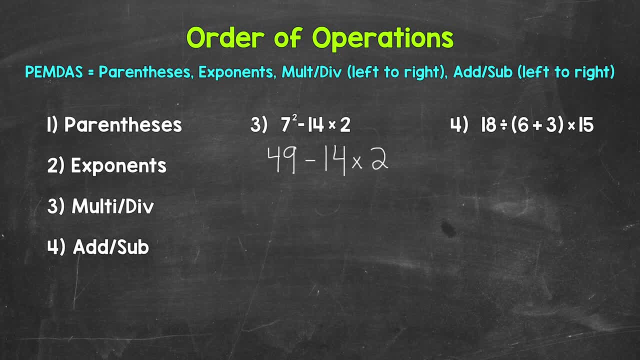 So now we have 49 minus 14 times 2.. Let's continue to work through the order of operations. Any parentheses, No, Any exponents, No, Any multiplication or division. Yes, we have multiplication, So that's what we need to do. next, We have 14 times 2,, which is 28.. Bring down. 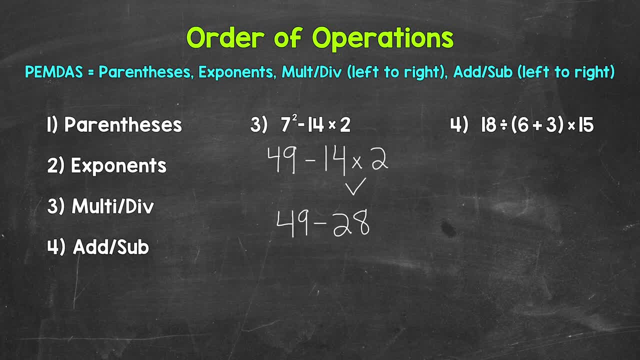 everything we did not use, And now we have 49 minus 14 times 2.. Let's work through the order of operations. Any so 49 minus 28.. We have one operation left- subtraction, so we need to subtract 49 minus 28. 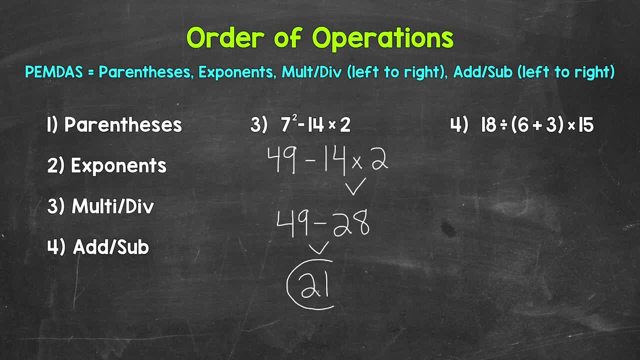 is 21.. So our final answer: 21.. Let's move on to number four, where we have 18 divided by, and then in parentheses, 6 plus 3, and parentheses times 15.. Let's work through the order of. 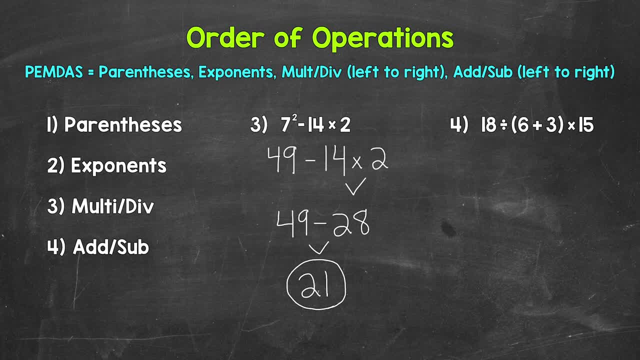 operations. Any parentheses in this expression: Yes, So we need to start there. We have 6 plus 3 in parentheses, That's 9, and then we need to bring down everything we did not use. So now we have 18 divided by 9 times 15.. Any parentheses: No. Any exponents: No Any.